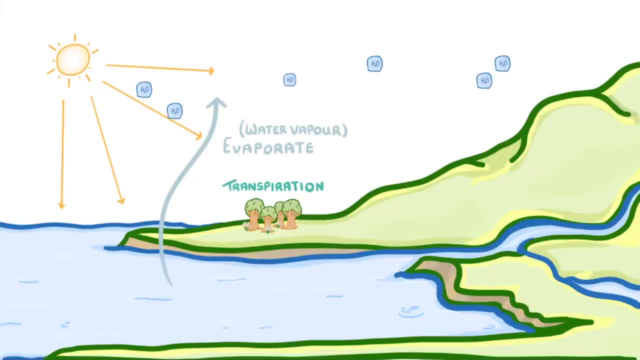 it into water vapour in the air. As all of this water vapour accumulates in the sky, it will start to condense into clouds, which can then be blown from one region to another, until at some point the water will fall back down to Earth as liquid water in the form of rain, which we call precipitation. 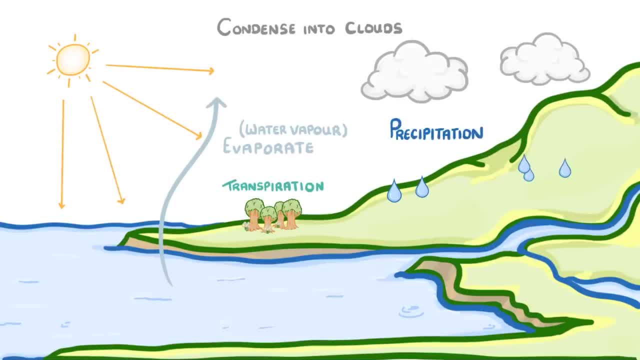 So now that the water has fallen back to Earth, it could seep into the soil, flow into rivers or be taken up by plants, And then this whole cycle can repeat all over again. Now the carbon cycle is a cycle. that is not just a cycle. The cycle is a cycle that is a cycle. 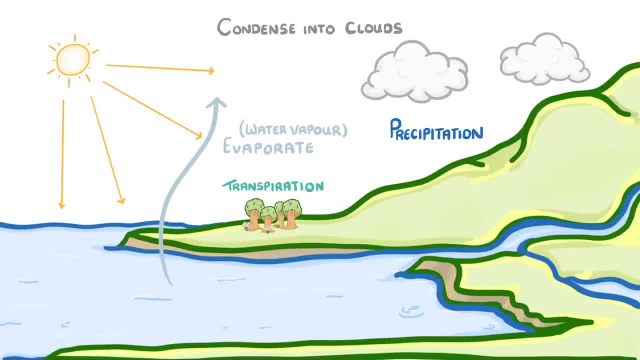 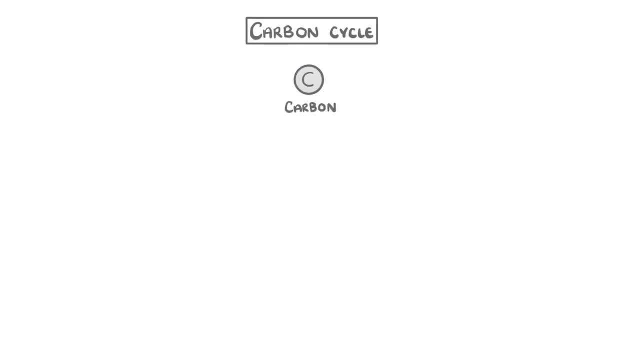 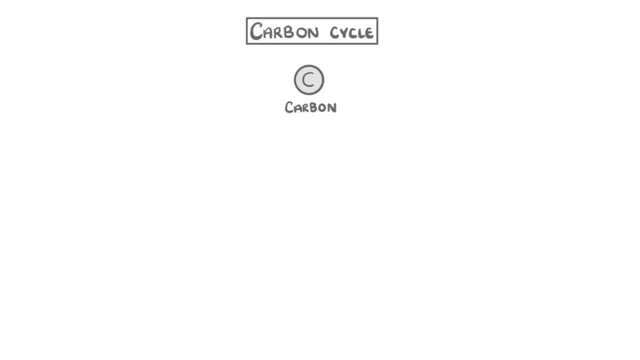 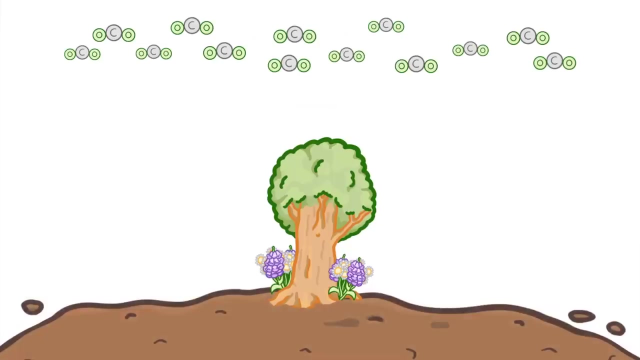 carbon is stored and then try to remember how it moves between them. Most of the carbon is split between 5 stores: In the air, where it's carbon dioxide. In plants, where it's locked up in biological molecules. In the soil, which contains lots of bacteria and other microorganisms. 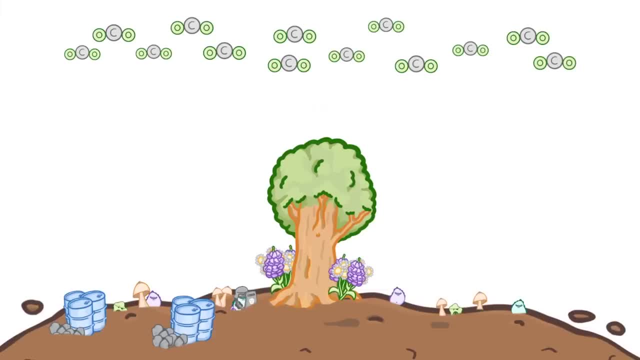 In fossil fuels, which are also underground, And, of course, in animals, where, like plants, it's locked up in biological molecules. So now that we know these different stores, let's look at how carbon moves between them. The most important process is photosynthesis, in which green plants and alga take in the 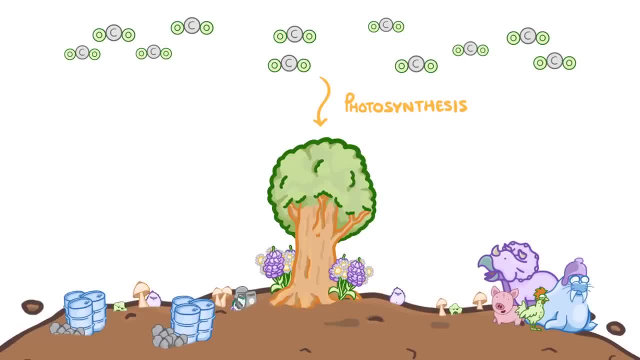 carbon dioxide from the atmosphere And convert it into biological molecules like glucose. This carbon that's now locked up inside them can then do two things: It can be passed back out to the atmosphere by respiration, Or passed on to animals that eat the plants. 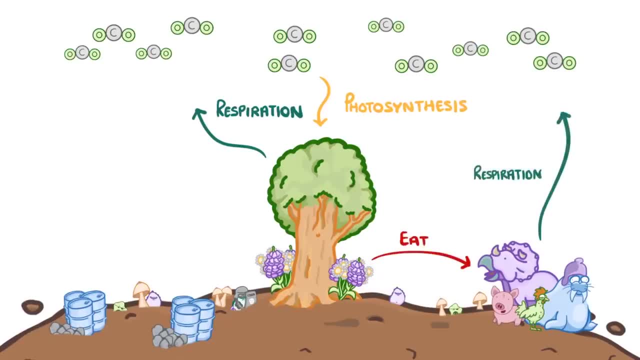 And, of course, the animals themselves could then also respire to release carbon dioxide. When these plants and animals die, though, two more things can happen to the carbon. One is that the organization of the carbon dioxide can then be transformed into the fossil fuels.